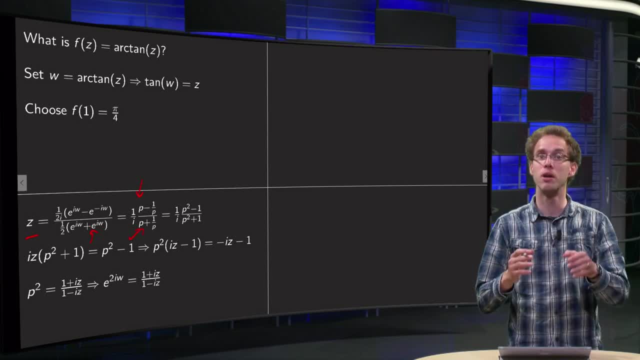 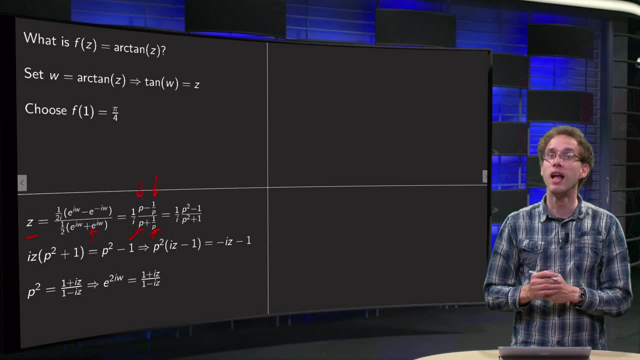 there. So e to the power minus i w becomes e to the power i, w to the power minus 1, equals 1 over p. So we get 1 over p over there, and over there then we multiply by p to get 1 over i p squared. 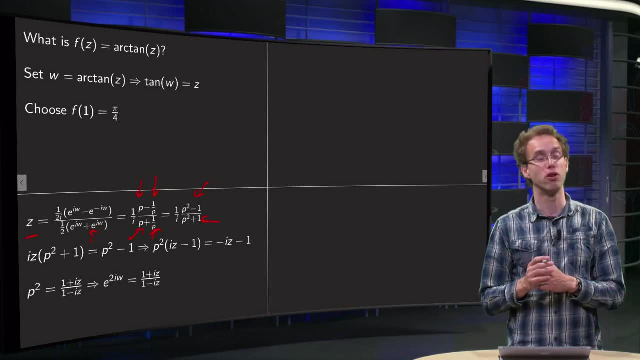 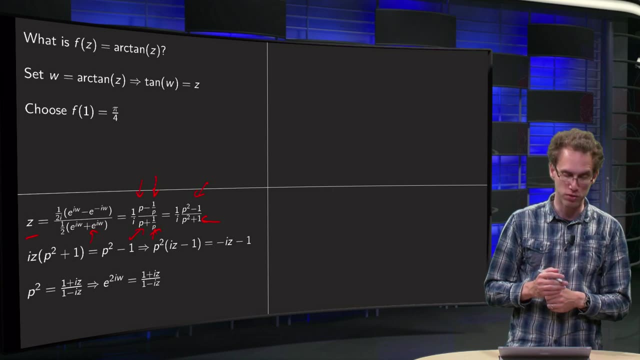 minus 1 over p squared plus 1.. Remember, we want to solve for w. p equals e to the power i w, so we can solve for p as well. so multiply by p squared plus 1 and by i, then we get p squared plus 1 times i. 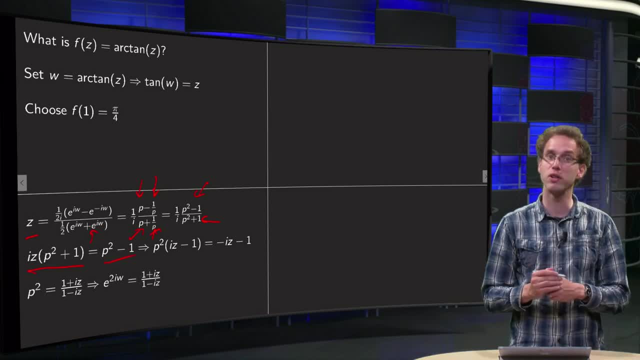 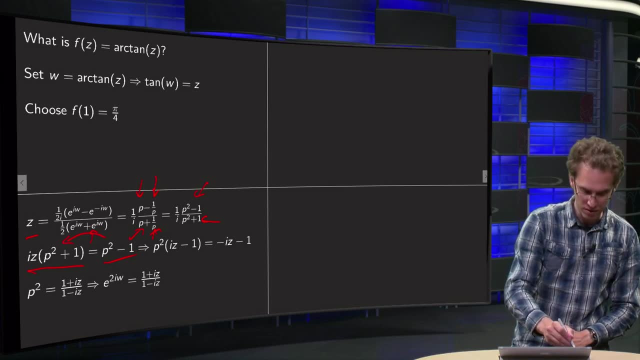 times z on the left hand side And we have only left the p squared minus 1 on the right hand side. we solve for p, so we bring the p squared to the left and the i z to the right, so we get the p squared. 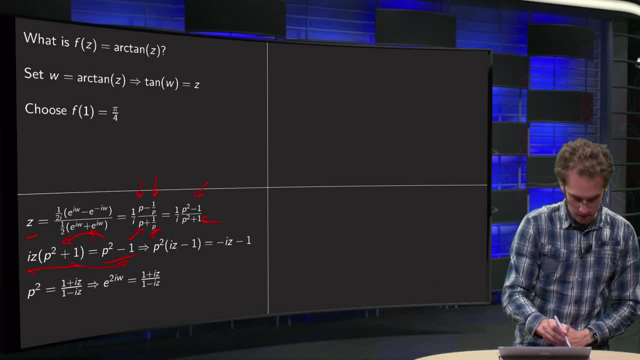 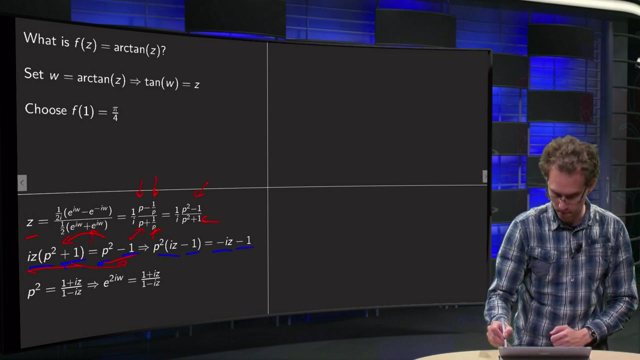 times i z over here, which we already had. we get a minus p squared from the other side. we get a minus 1,, which we already had, and we get a minus i z from the left hand side over here, And then we can divide by i z minus 1, so we get a p squared equals minus. i z minus. 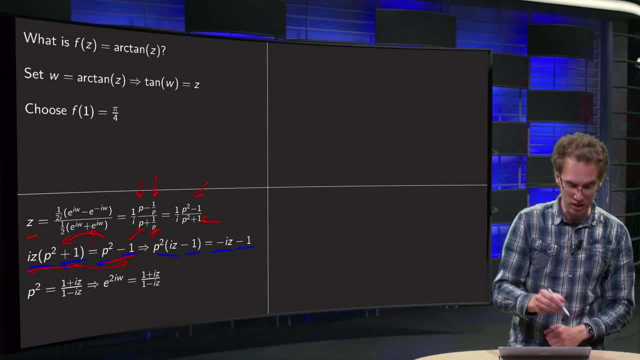 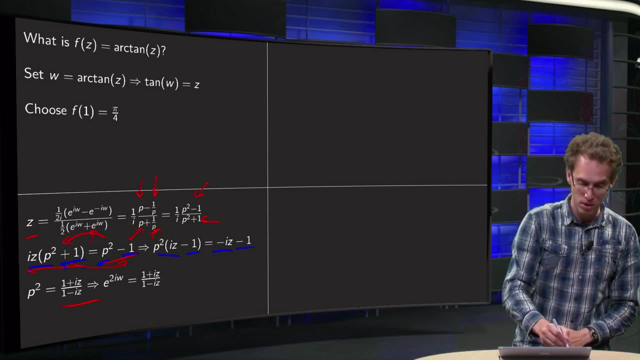 1 divided by i z minus 1, and take out the minus signs: 1 plus i z over 1 minus i z. And remember p was e to the power i w, so p squared equals e to the power 2 i w, so 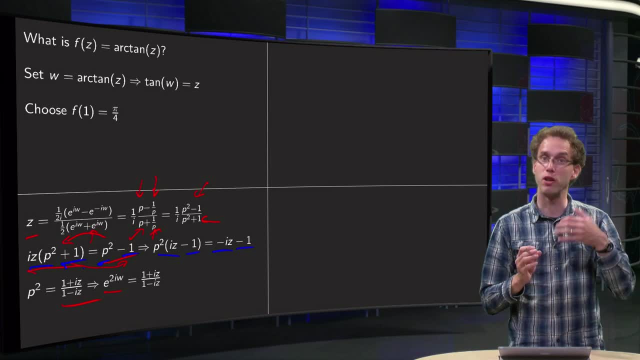 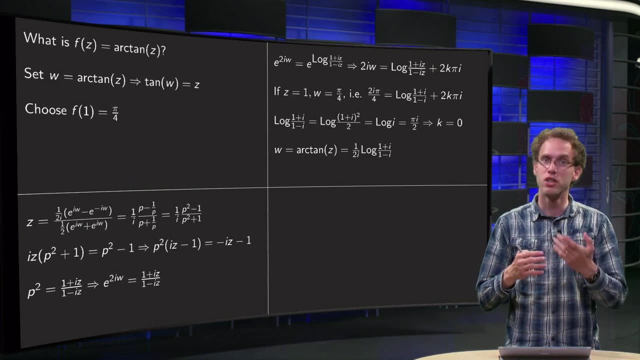 we almost have our w in terms of z And we only have this exponential and we have to be a bit careful when taking logarithms. so we set on the left hand side we just leave the e to the power 2, i w on the right hand. 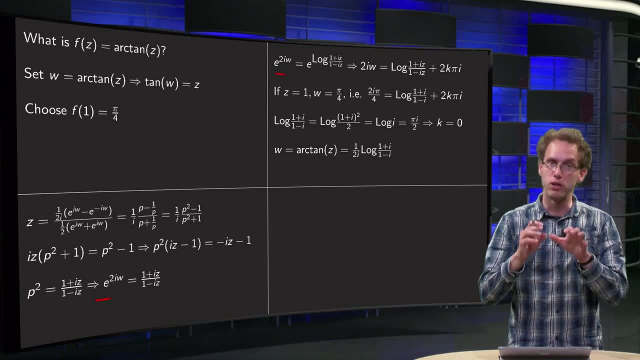 side. we turn this in the exponential as well. the rubbish equals e to the power log of the rubbish. so there we are, And then we cancel out the exponentials. If we take into account this fraction, 2k, pi, i, then the e to the power, i equals e to. 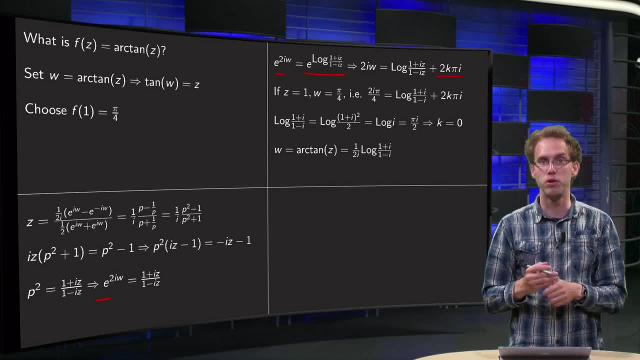 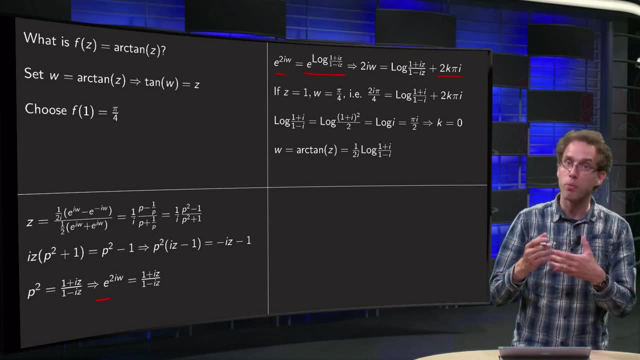 e to the power of b is a, and then a equals b plus e to the power of 2 pi i, because e to the power of 2k pi i equals 1.. So now we can almost solve for w, but we want to know our k, on which branch we are. 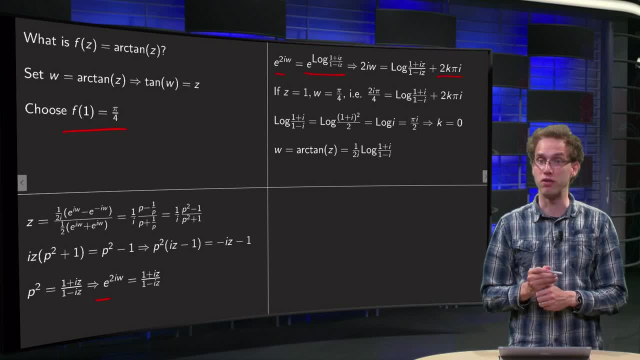 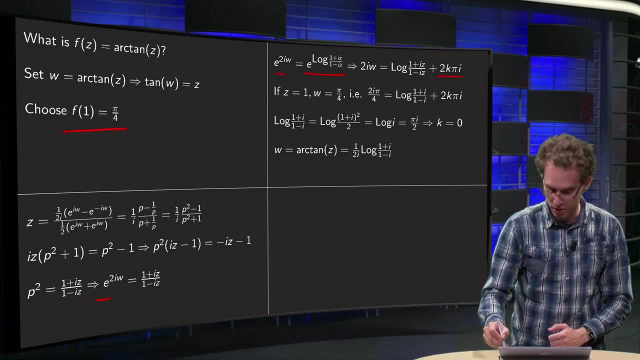 For that we use our condition f of 1 equals pi over 4, so we plug in z equals 1 and we plug in w equals pi over 4, and that will yield our k. that will tell us which value of k we have to choose. 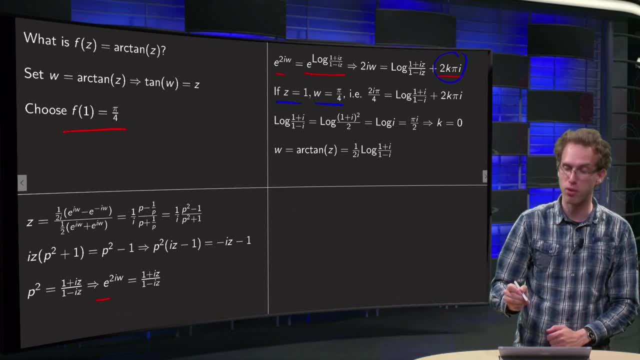 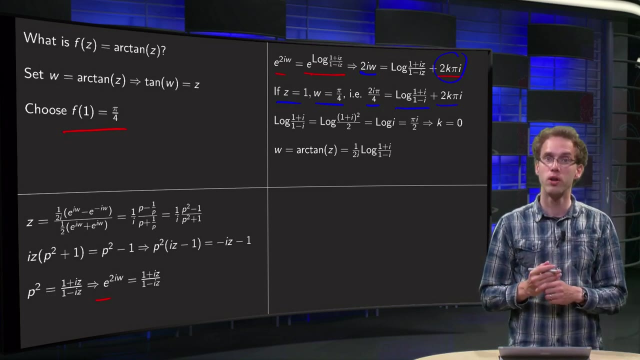 So we set 1, w equals pi over 4, so this 2i w becomes 2i. pi over 4 equals the log of 1 plus i over 1 minus i plus 2k pi. i Simplify this log by multiplying by 1 plus i numerator and denominator. 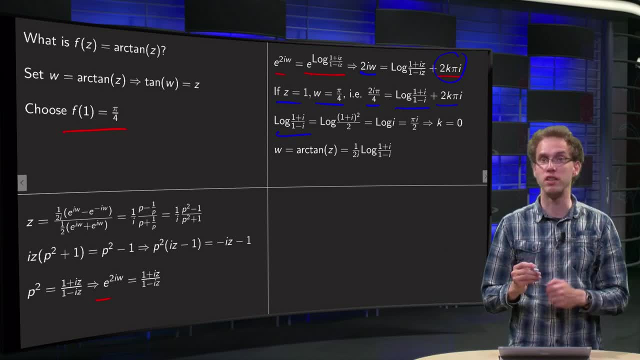 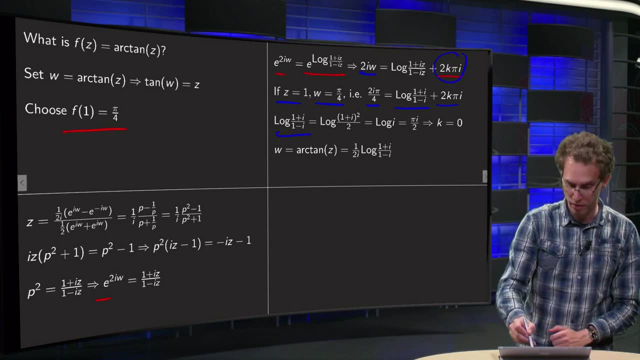 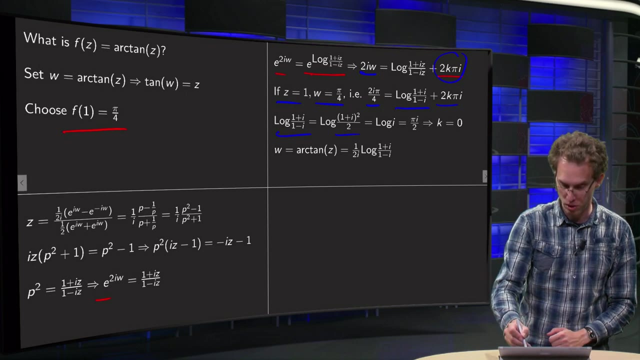 So our log becomes 1.. 1 plus i squared in the numerator and 1 plus i times 1 minus i equals 1 minus i squared equals 1 minus minus 1, so two over here, and 1 plus i squared equals 1 plus 2i plus i squared equals. 2i over 2 equals the log of i. 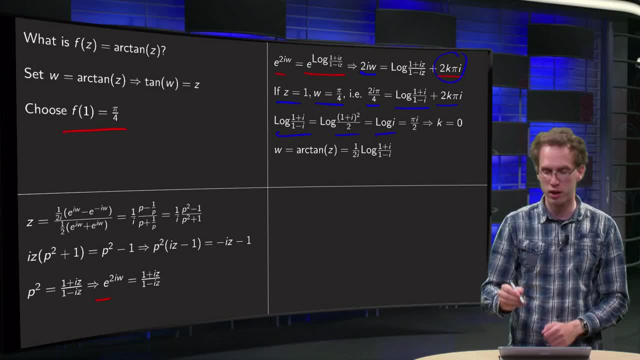 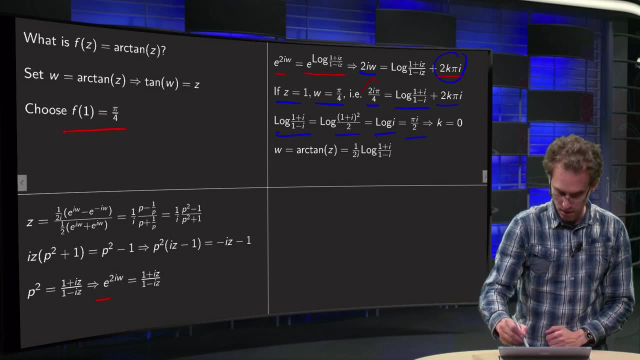 It is e to the power of ln of 1 plus i times the argument: so pi over 2.. So now we see that the pi over 2 which we have over here equals the log over 1.. letter f and that becomes 5. there is 4 in the numerator. 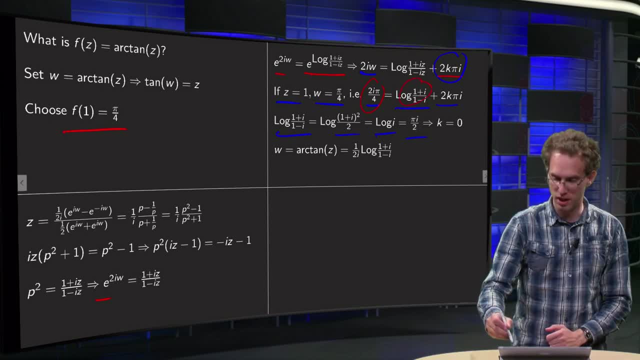 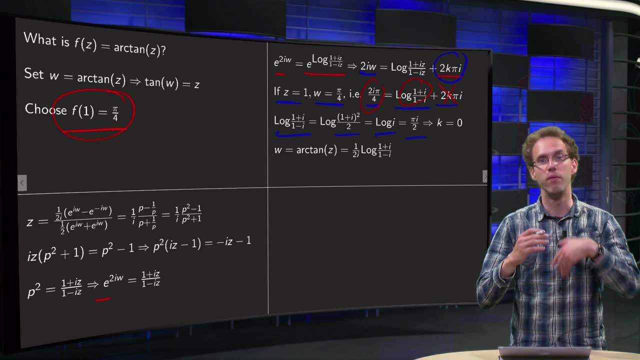 log of i equals pi over 2 over here. so that means that this k has to be 0, that means that time has to vanish. This our choice, due to our choice over here. with another choice we would have another value of k. 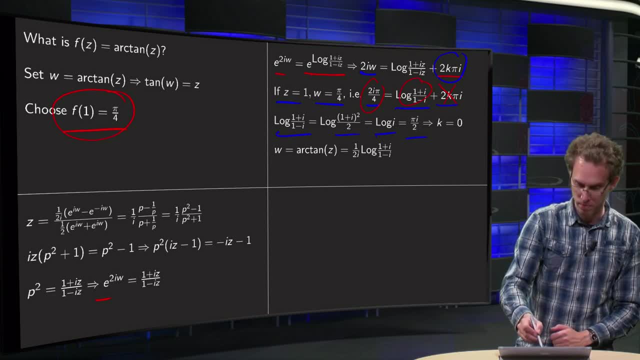 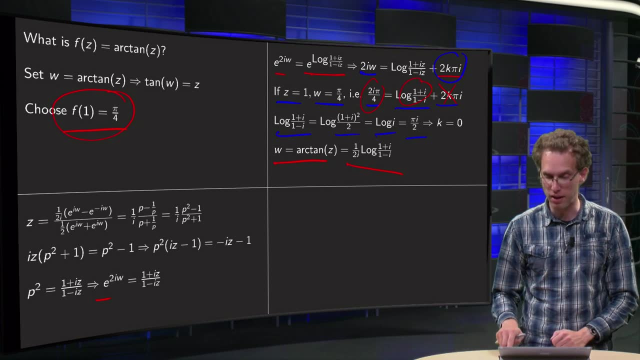 And then we conclude that w equals the arctangent of z equals this log divided by 2i. You know, if you have a log you have to be careful of branch points and branch cuts. so where are the branch points and the branch cuts for the arctangent? 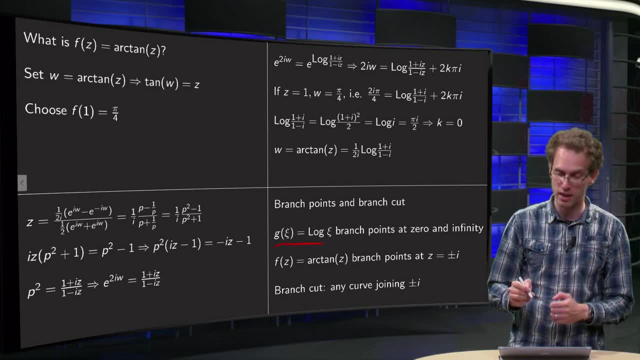 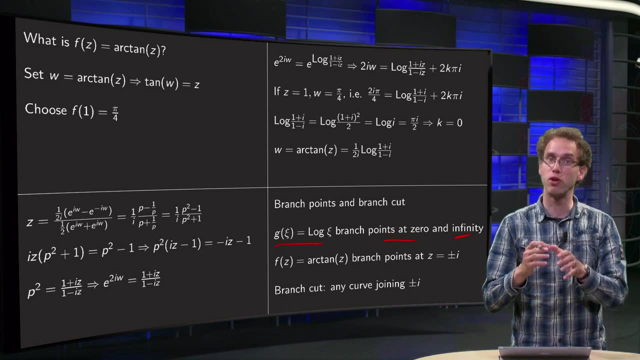 Well, if you have a function g of xi equals the log of xi, your branch points are at 0, at infinity, that's known. So where are your branch points now? Well, when the argument of your log is either 0 or infinity. so when is this 0 or infinity? 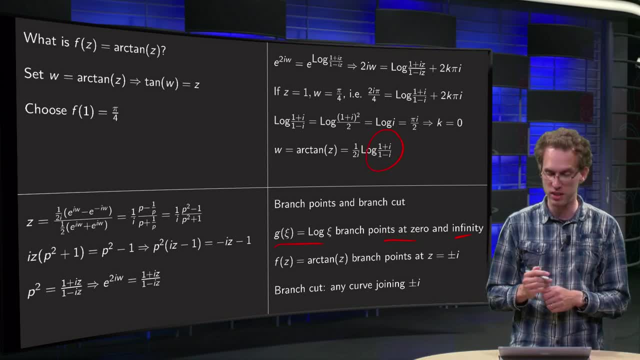 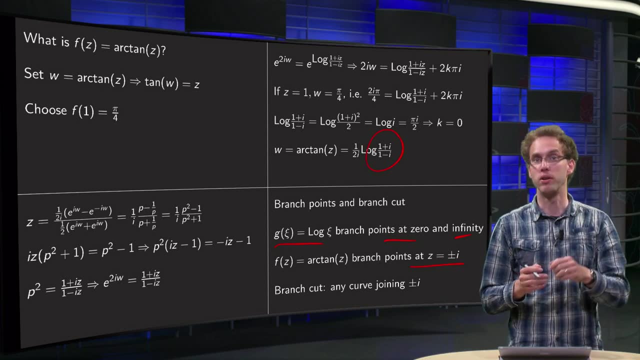 Well, at minus i, you are at 0,. at plus i, you are at infinity. that means that your branch points will be at plus or minus i. and for a branch cut, well, you can choose any of them, Any curve joining plus or minus i.